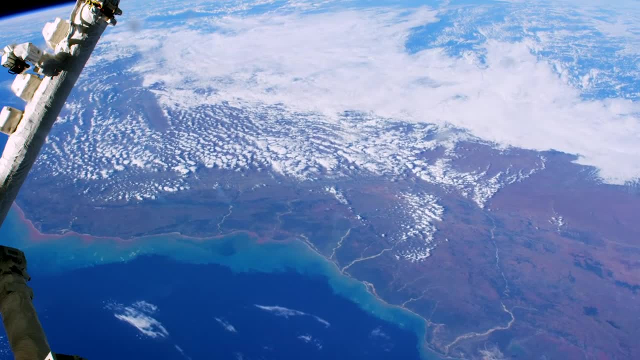 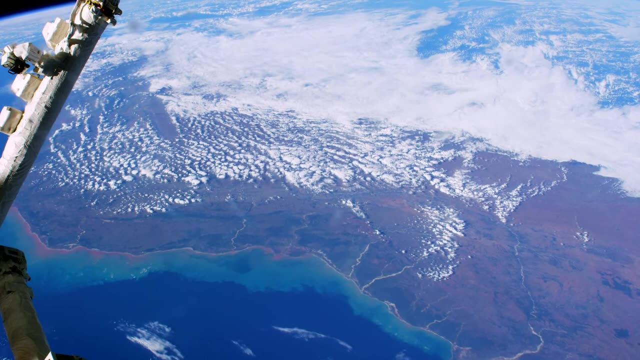 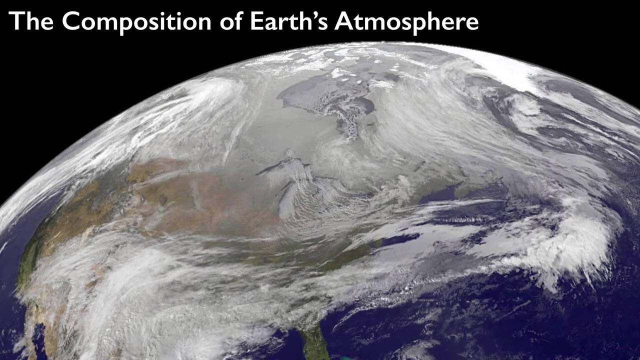 of the Earth's atmosphere. However, it is important for you to have a sense of scale for the planet you live on and the vital nature of those first few kilometres of air. The examiner will ask you about the composition, The composition of today's atmosphere, which is a mixture of three main gases. You need to know. 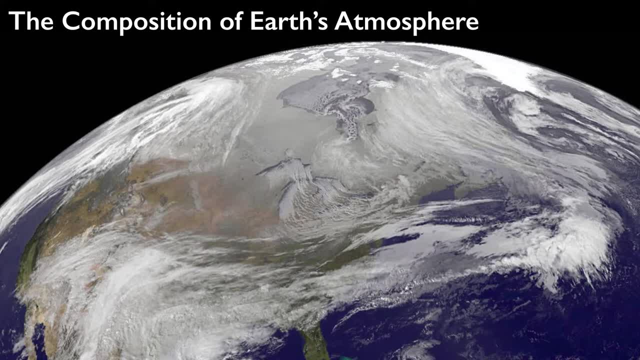 their names and the percentages of each one. The composition may surprise you. First of all, the most common gas by far is nitrogen and not oxygen. Discounting any water vapour that we might find, our air is approximately 78% nitrogen. The next most common is oxygen, at 21%. 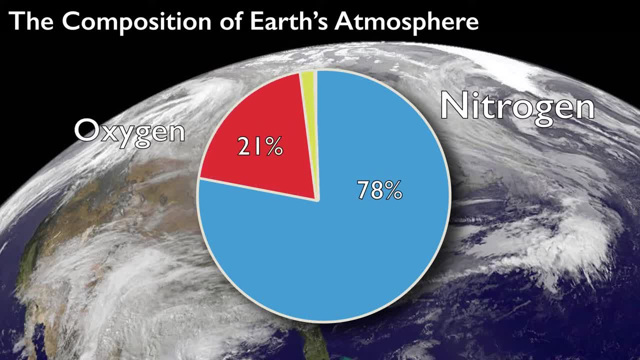 and the last 1% is mainly the inert gas argon. Now you hear quite a bit about carbon dioxide in the news and of course it's carbon dioxide that we breathe out, that plants require for photosynthesis and that we release when we burn fossil fuels. But in actual fact, 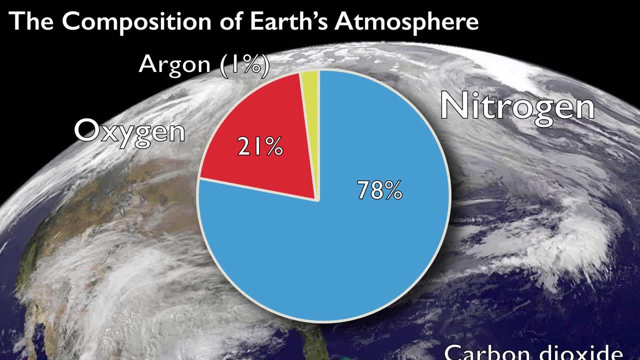 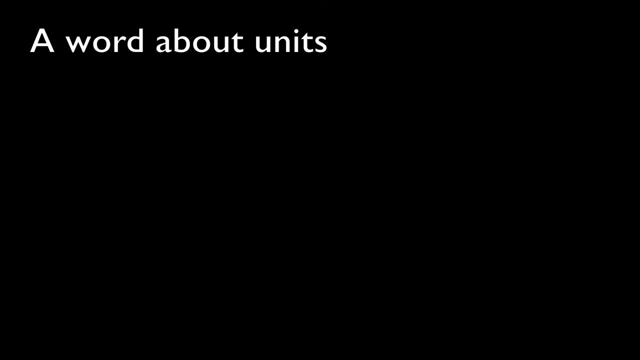 carbon dioxide makes up only 0.04% of our atmosphere. Thinking about that 0.04%, we should talk about some of the most important information about the environment. The most important briefly, about units. Scientists and examiners may use another unit. 1% is the same as saying: 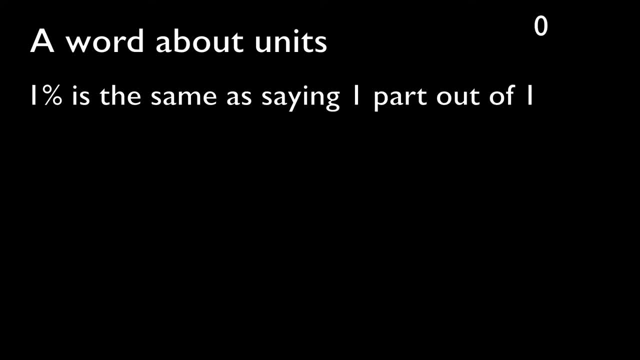 one part out of 100. And so 0.1% would be the same as one part out of 1000. And 0.01% would be the same as one part in 10,000.. The examiner will talk about parts per million, And so 0.04%. 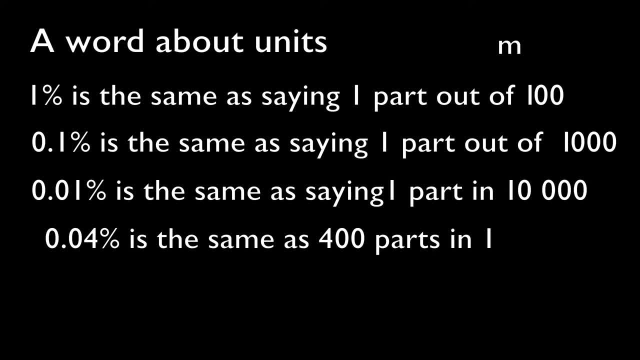 is the same as 400 parts per million, or 400 ppm as it gets written down. Now you won't be asked to convert between percentages and parts per million, certainly not without the examiner Giving you a formula. But you do need to be aware of this unit as it might turn up in. 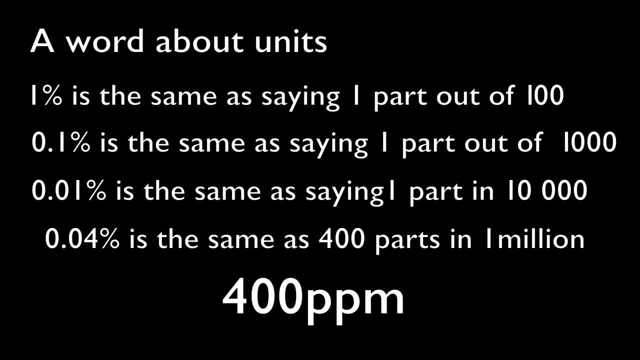 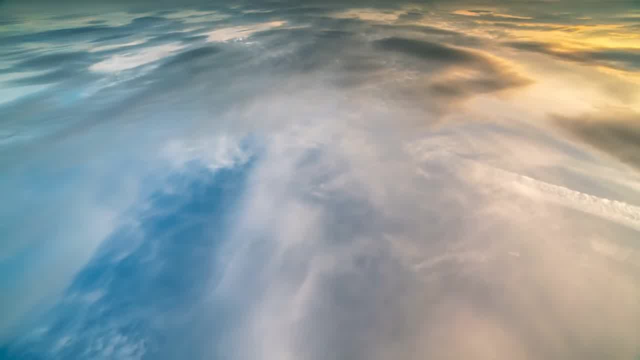 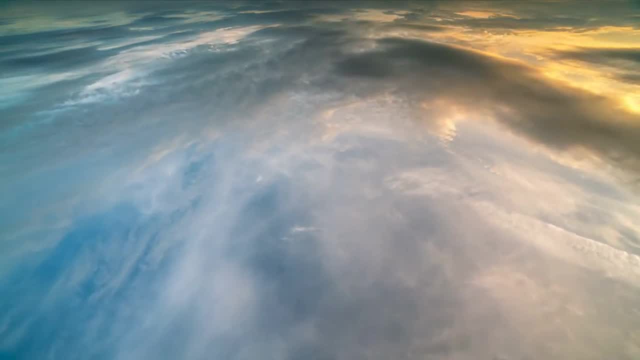 tables, graphs, charts or in the text of an exam question. There are also other gases in our atmosphere, principally the remaining inert gases. Neon, helium and krypton all make up tiny amounts of it, along with about one to two parts per. 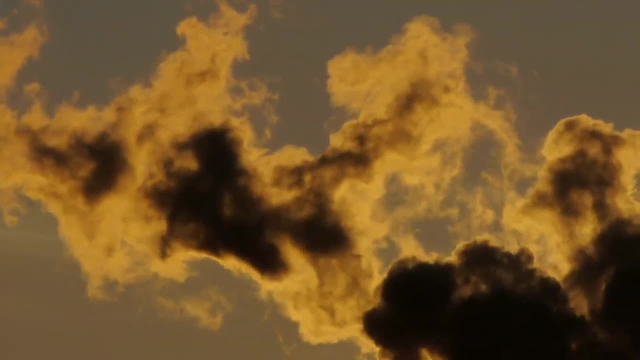 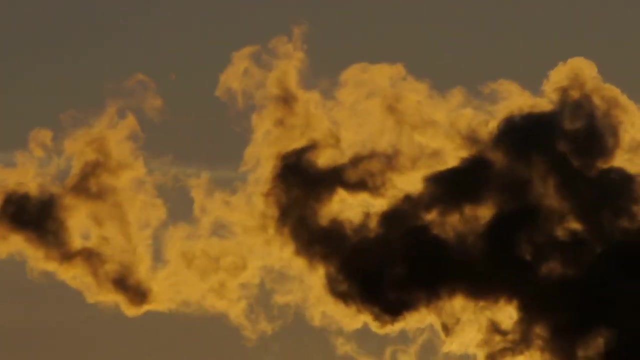 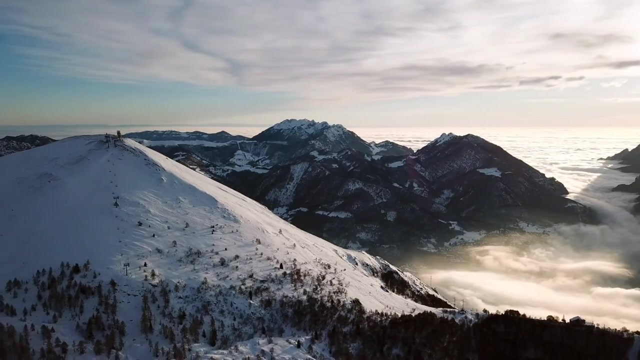 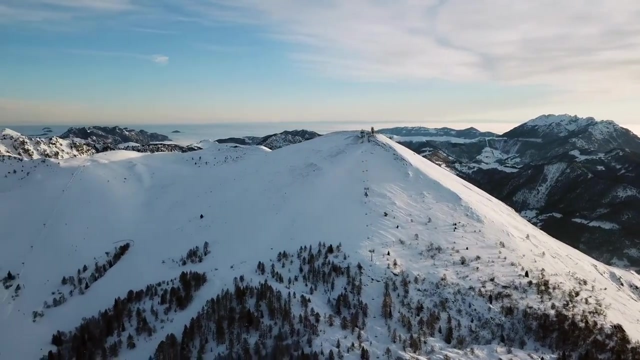 million of naturally effective gas. Other gases are generally referred to as pollutants and we'll talk about them in later lessons. So this is the air we breathe And, despite the fact that human activity and atmospheric pollution has made some changes to the atmosphere over the last few hundred years, the actual size of those changes relative to the main gases in the atmosphere are tiny. In fact, the percentages of the common gases in our atmosphere have hardly changed at all for the last 200 million years, And that's all the way back to the time of the early 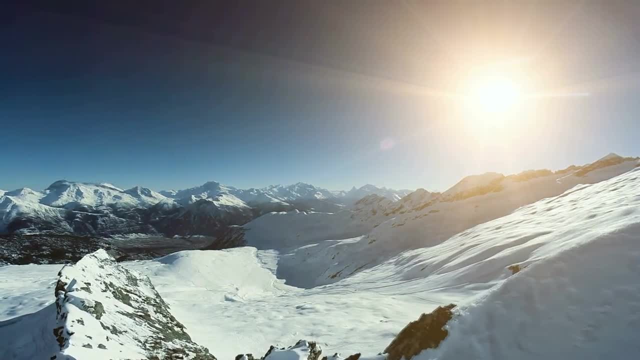 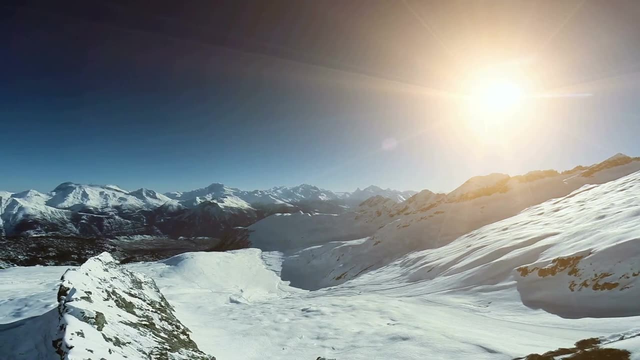 dinosaurs. The examiner quotes the following basic figures: That for the last 200 million years, our atmosphere has been approximately four fifths nitrogen, That's around 80%, And one fifth oxygen, That's 20%, And small proportions of other gases, notably carbon dioxide, water vapor and the noble 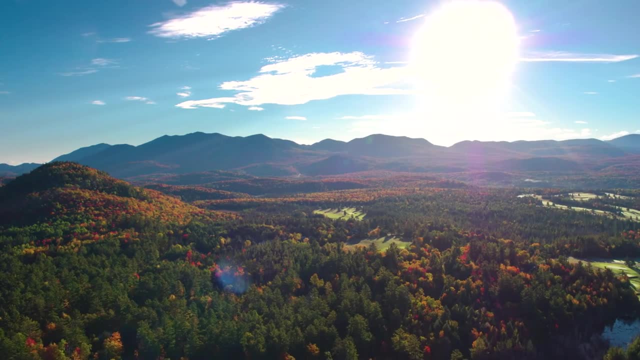 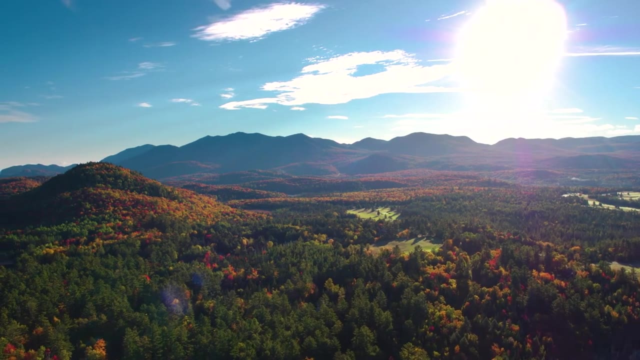 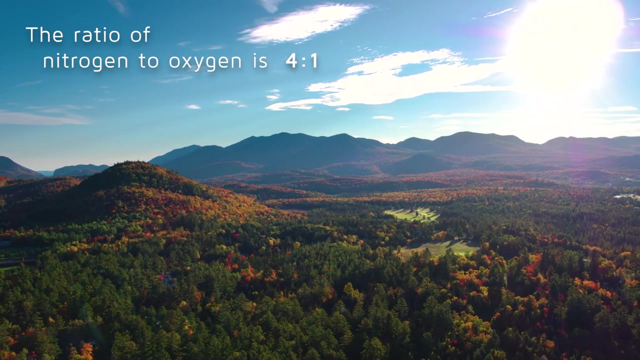 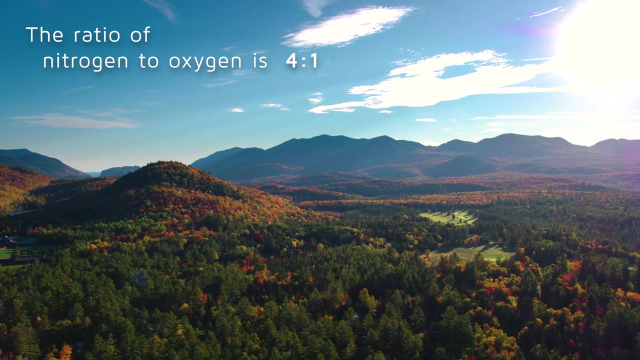 gases. The examiner could choose to use fractions, percentages or even ratios in their questions. So it's also worth noting that the ratio of nitrogen to oxygen is pretty much 4 to 1.. You should make sure now that you can recall the percentages of the gases in the atmosphere. 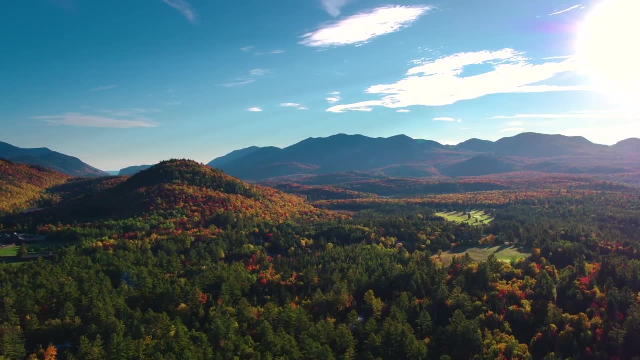 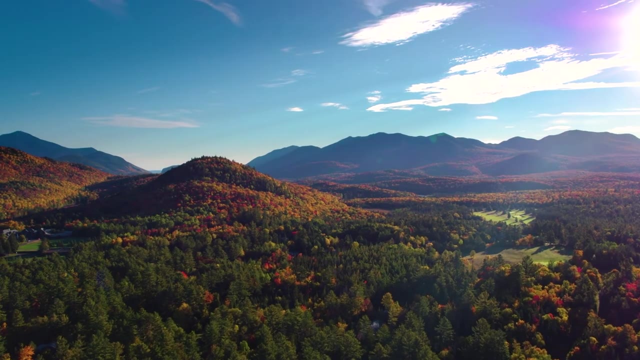 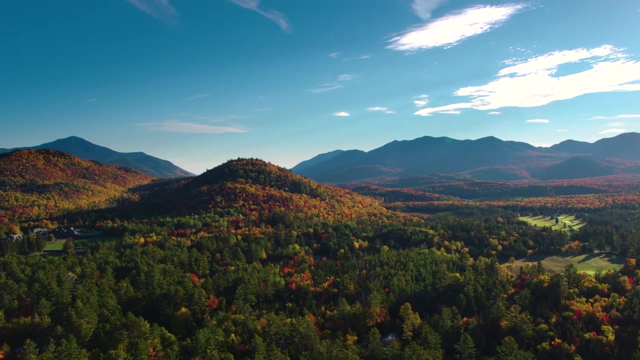 and be familiar with those numbers as percentages, ratios, fractions and also parts per million for the rarer gases. Take some time now and learn those off by heart, so it will be easy marks to get in the exam. In the next lesson we'll be looking at where our atmosphere has come from. 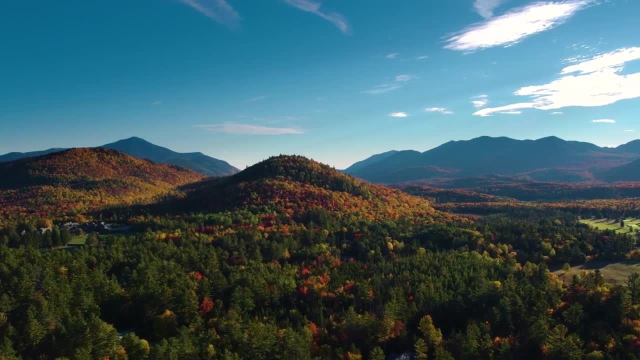 and we'll be taking you right the way back to the early days of our planet to explain its origins.